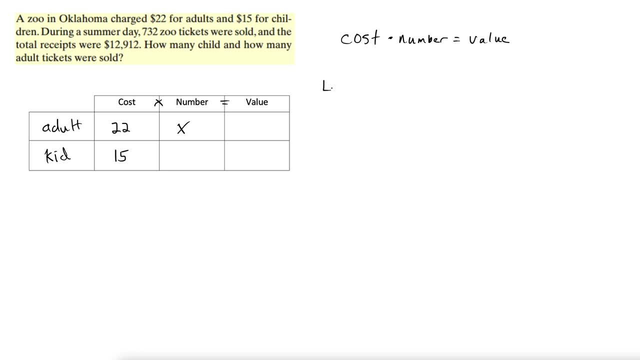 let's let that be x, Alright, so just remember that. Let x be the number Of adult tickets Sold, Alright. and Now we're only using one variable right now, So the number of kids tickets sold. Let's see, here We had $732 total. Well, if x were the adult number, the 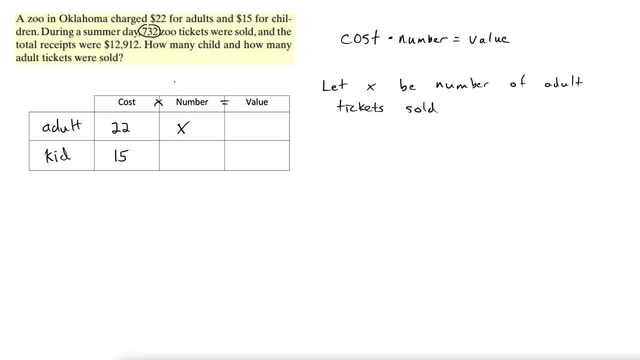 number of adult tickets? I don't know, I don't remember. I think I got this one wrong, I don't. then the rest must be the number of kid tickets. So how do we represent the rest mathematically? Like this: 732 minus x. 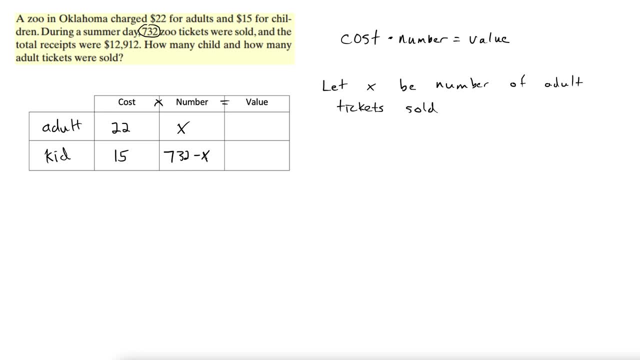 Okay, I took the total number of tickets sold. I subtracted off the adult tickets. that gives us the kid tickets. There's only adult and kid tickets sold period, so the rest of them must be the kid tickets. Alright, multiply across, we get 22x. 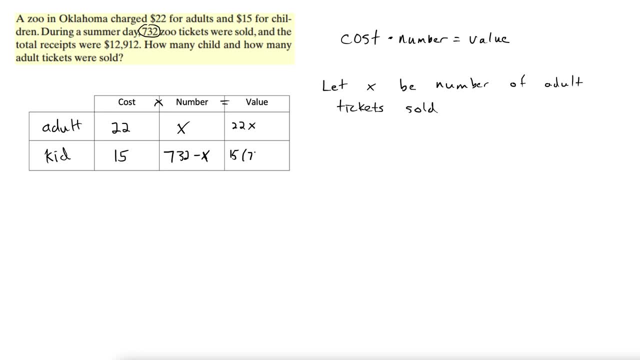 and down here we get 15, 732 minus x The value. how much money did each of these bring in? Well, the total value comes from right here: 12,912.. So we add these two up to get the total value. 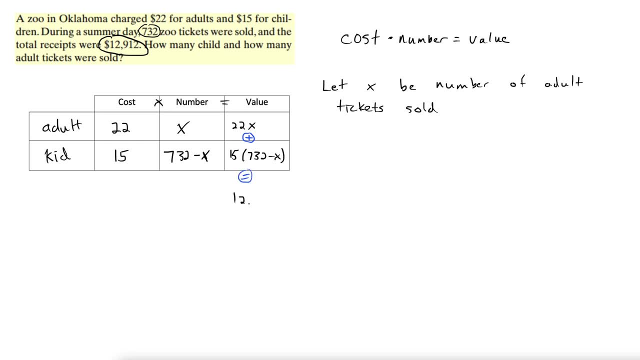 that number comes to 12,912.. And this column, this column right here, gives us the equation we need to solve the problem. So let's pull that from the table: 22x plus 15, 732 minus x equals 12,912.. 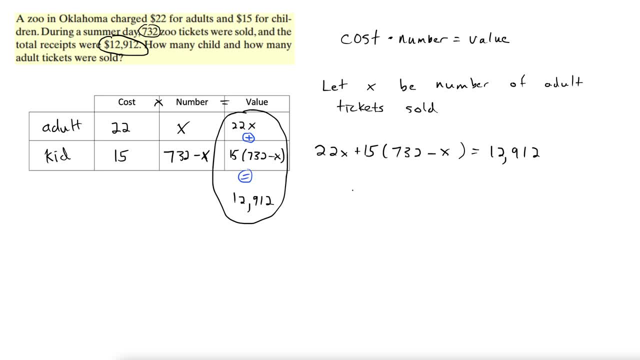 Okay, now we just have to solve this equation. Not entirely trivial, but the hard part is done. Let's distribute this 15, we get 22x plus. let's see 15 times 732.. Need a calculator for that.